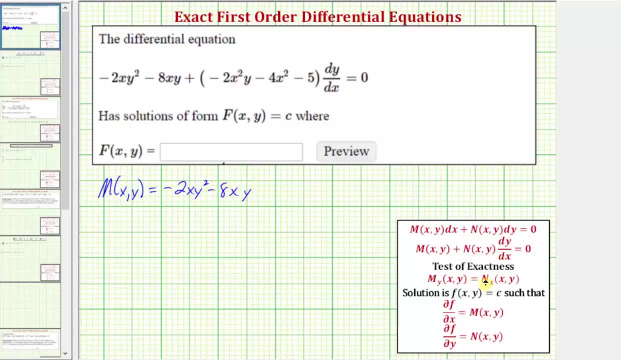 And n of x comma y equals negative: 2xy squared minus 4x squared minus 5.. So for our next step, let's verify: these partial derivatives are equal. So now we'll find the partial of m with respect to y. So we'll differentiate m with respect to y, treating x as a constant. 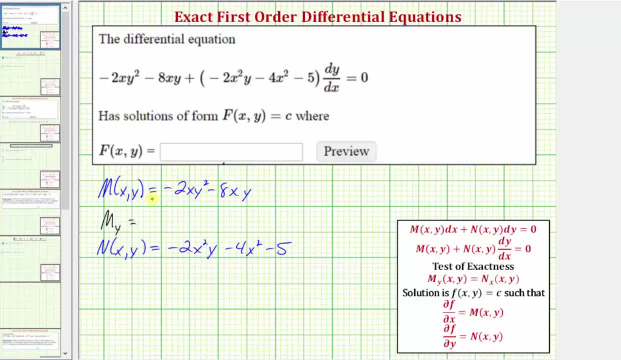 So the derivative of negative 2xy squared minus 4x squared minus 5.. The derivative of negative 2xy squared with respect to y would be negative 4xy, And then we'd have minus. the derivative of 8xy with respect to y would be 8x. 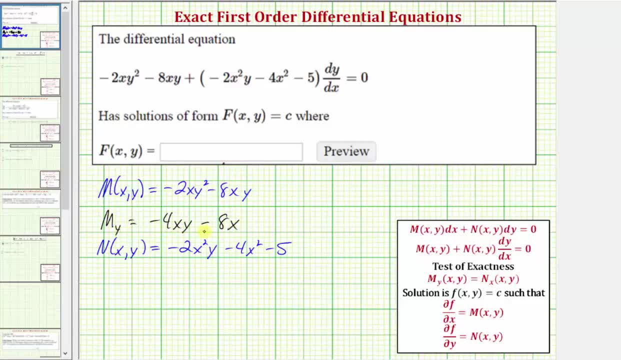 So the partial of m with respect to y is negative 4xy minus 8x. Now let's find the partial of m with respect to x, which must equal negative 4xy minus 8x if this is an exact differential equation. 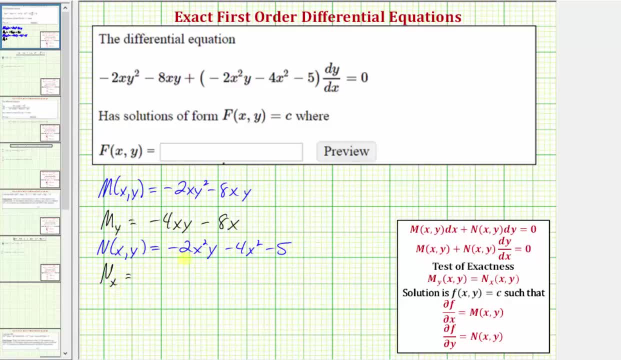 So we'll differentiate m with respect to x, treating y as a constant. So the derivative of negative 2xy squared minus 8x With respect to x would be negative 4xy, And then we'd have minus. the derivative of 4x squared with respect to x is 8x. 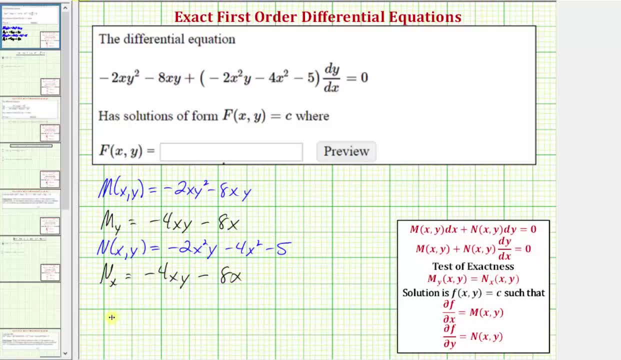 And then the derivative of negative 5 would be 0. So notice how the partial of m with respect to y does equal the partial of n with respect to x, And therefore we do have an exact differential equation. So the solution to the exact differential equation. 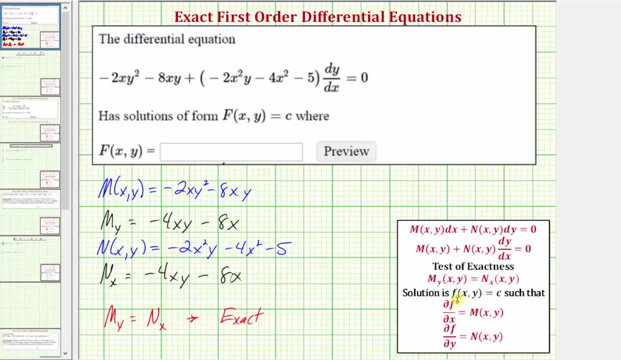 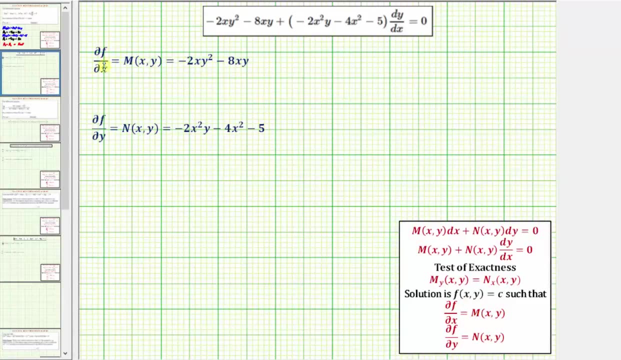 would be: f of x comma y equals c, such that the partial of f with respect to x equals m and the partial of f with respect to y equals n. So now let's work on determining the function f of x comma y. So this first equation here tells us: the partial of f with respect to x must equal m. 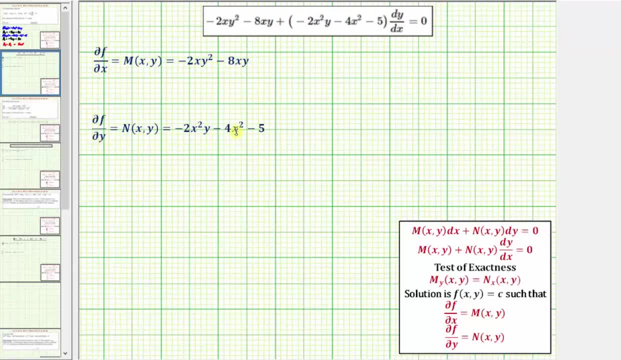 and the partial of f with respect to y must equal n. So to recover the function f of x comma y, we integrate m with respect to x. So f of x comma y is equal to the integral of m, which is negative 2xy squared minus 8xy integrated with respect to x. 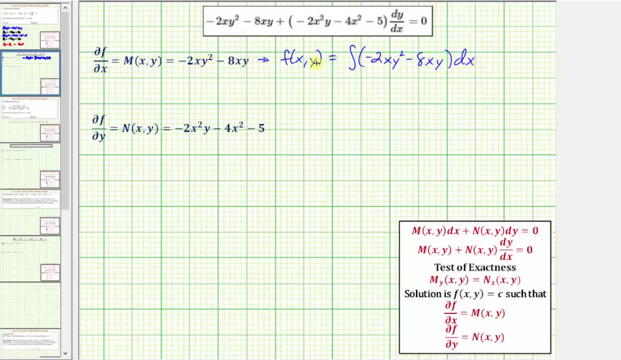 But because we're integrating with respect to x, we are not going to recover the y terms of f of x comma y, So we'll have to include plus a function of y when integrating. So f of x comma y is equal to the integral of negative 2xy squared with respect to x. 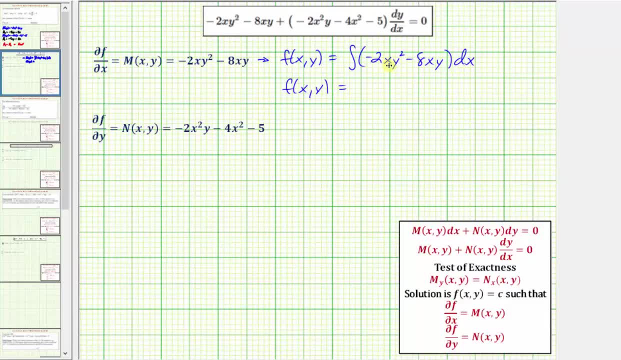 would be negative 2y squared times y squared divided by 2, which would give us negative x squared y squared minus the integral of 8xy with respect to x, which would be 8y times x squared divided by 2.. So we have minus 4x squared y. 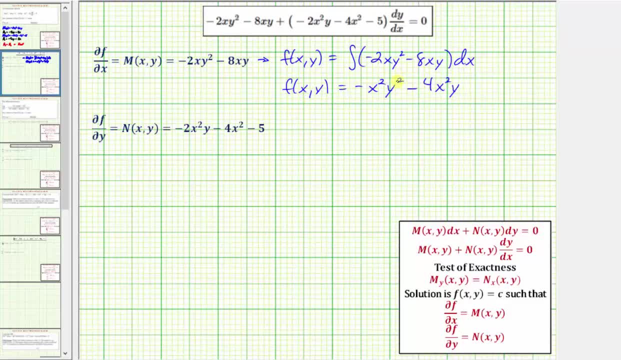 And again we're not recovering the y terms of f of x comma y, So we'll have to write plus a function of y. Let's write plus h of y. Now we also know the partial of f with respect to y must equal n. 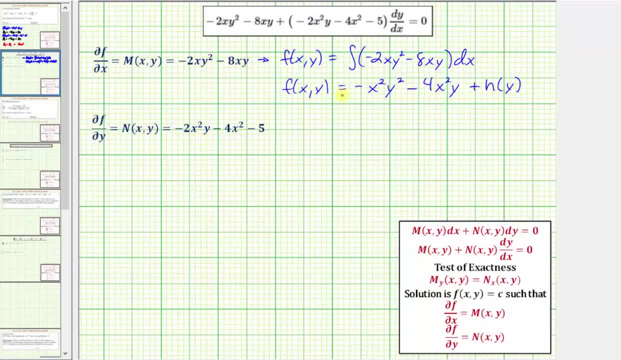 Which means if we differentiate f of x comma y, which we just found, with respect to y, it must equal n of x comma y. So this must be equal to, again, the partial of f with respect to y. So we'll differentiate with respect to y. 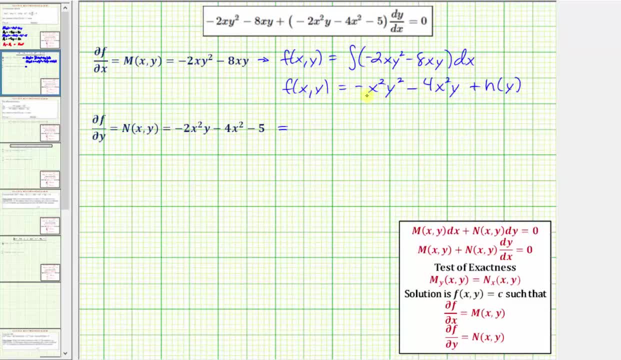 treating x as a constant. So the derivative of negative x squared y with respect to y would be negative 2x squared y. And then we'd have the derivative of negative 4x squared y with respect to y, that'd be minus 4x squared. 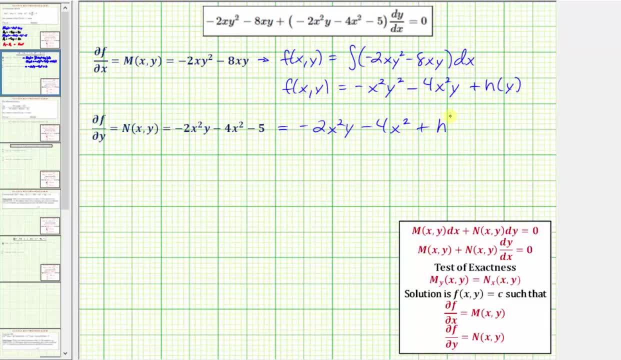 plus the derivative of h with respect to y would be just h prime of y. Now we want to compare the terms of the partial of f with respect to y to n of x comma y. Notice how we have negative 2x squared y. 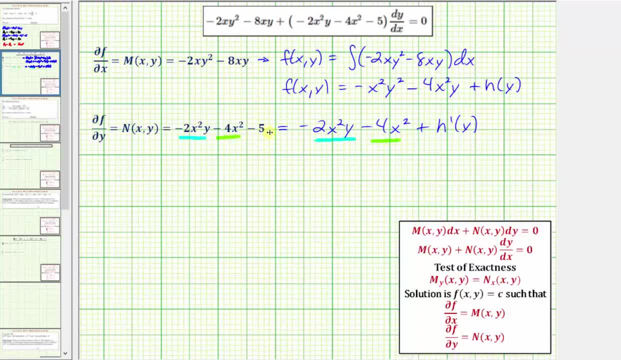 We also have negative 4x squared, But notice, here we have the term negative 5, and here we have h prime of y. So this tells us h prime of y must equal negative 5.. So if h prime of y equals negative 5,, 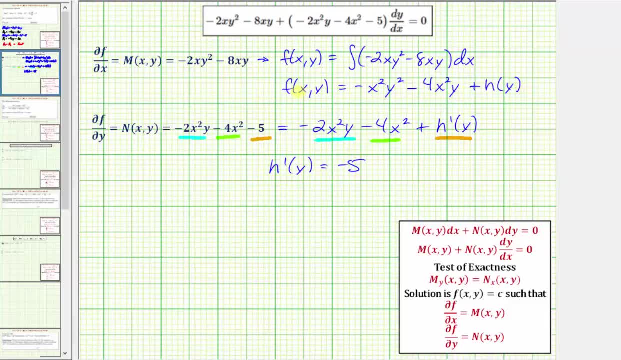 if we can find h of y, we can determine the function f of x comma y. So to find h of y, we'll integrate both sides of this equation. So we'd have the integral of h prime of y. dy equals the integral of negative 5 dy.